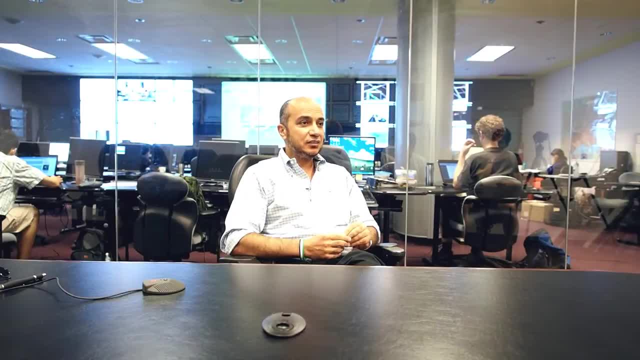 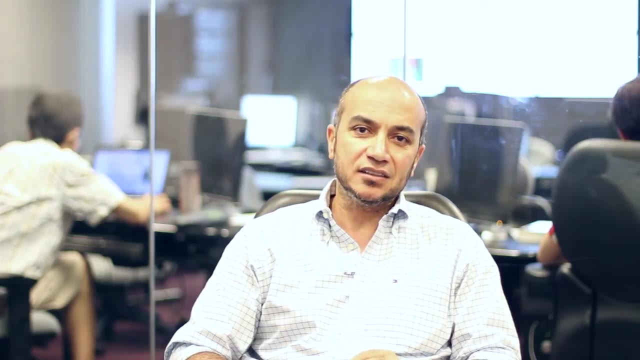 the most cutting-edge topic is as fresh as today. Today, we just graduated a brilliant PhD student. She developed a system that makes traffic lights learn. So think of a traffic light as a robot, for example, where as it sees congestion develop and as it tries different combinations of control strategies. 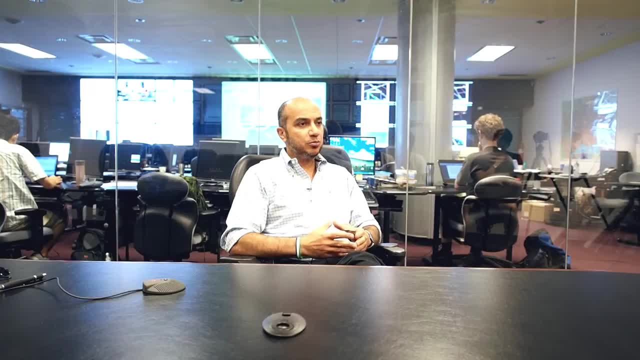 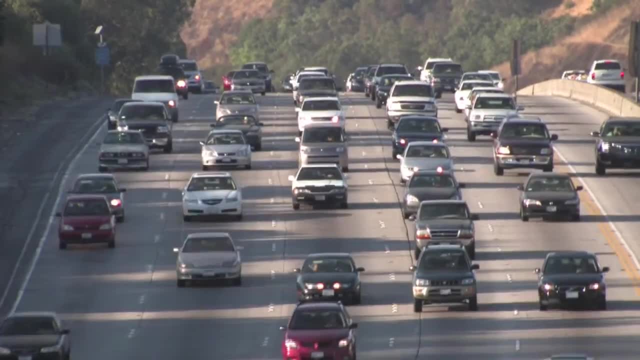 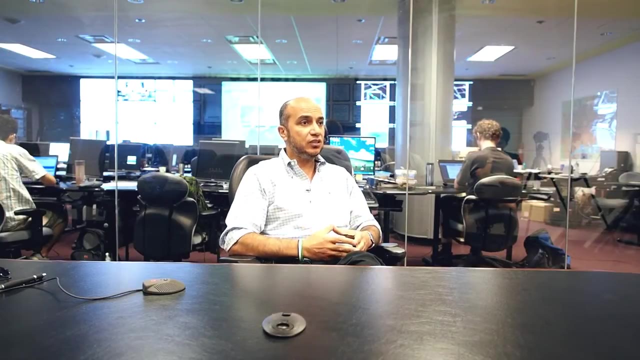 it would learn what works and what doesn't work. Transportation problems are household problems. nowadays. You don't need a PhD to realize that there's congestion and the transportation system is breaking down. So everybody suffers in traffic- Everybody. even if you take, transit still is not as fast as we would like it to be. 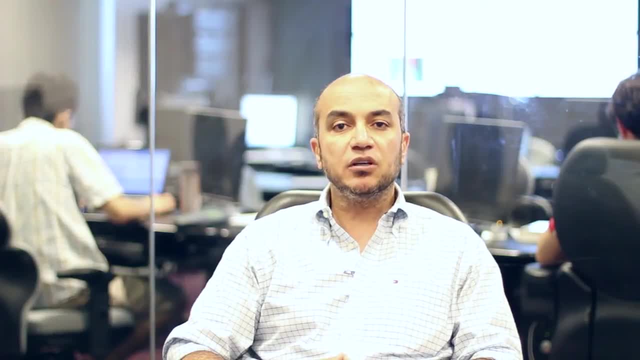 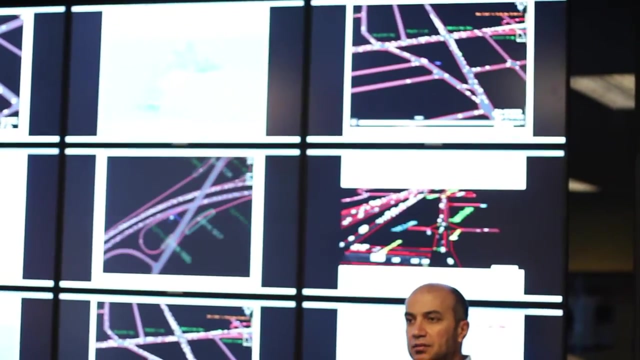 We collaborate with a number of stakeholders For the government, for example, where we're at at the moment at the ITS Center at U of T. this research center is connected to hundreds of cameras and several hundred detectors that measure traffic congestion in different places in the Greater Toronto Area. 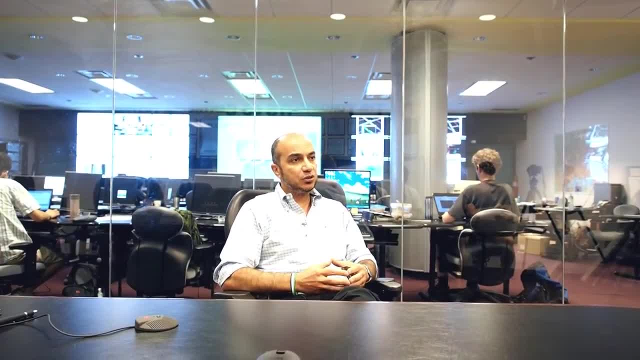 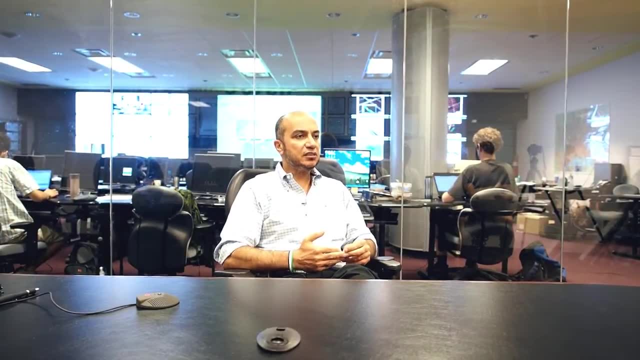 And these are owned and operated by the Ministry of Transportation of Ontario and the City of Toronto. But rather we use what we see for research and development. So our masters and PhD students use the information to come up with creative solutions to transportation problems. 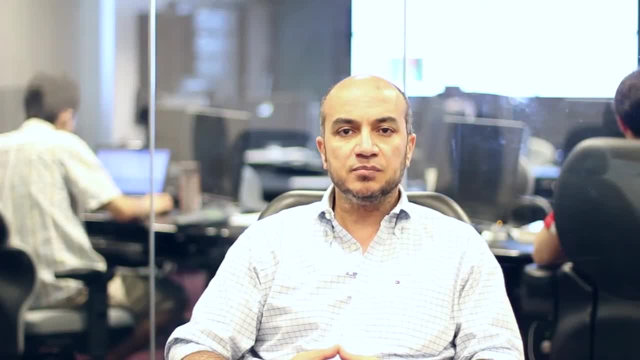 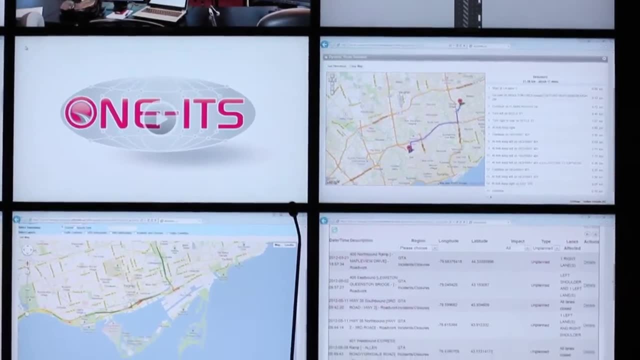 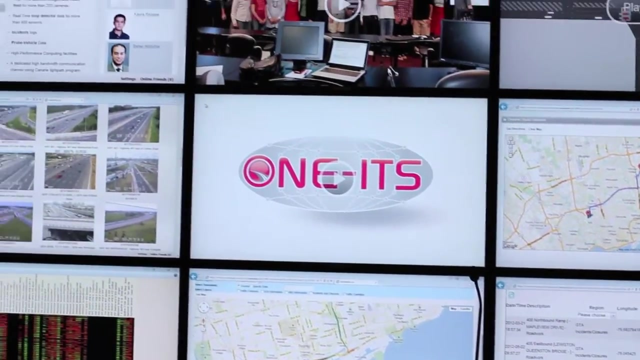 Now we also have systems that connect universities across Canada to this center, OneITSnet, which is the web-based platform that we have, And you have access to information from Toronto. You can test your systems on Toronto Or you can lend us whatever you're doing at the University of Calgary or any other university. 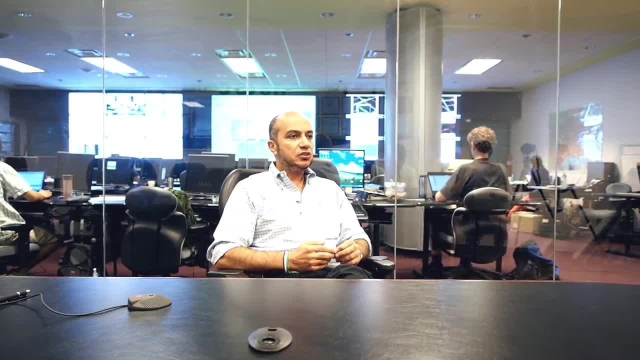 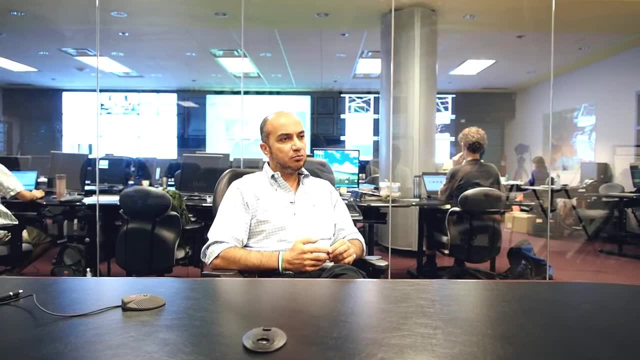 The future of intelligent transportation systems. I can think of it as threefold. The first thing that we'll see is much more efficient transportation networks. For instance, you receive information on your smartphone telling you where congestion is and where else has spare capacity, so you can avoid congestion.